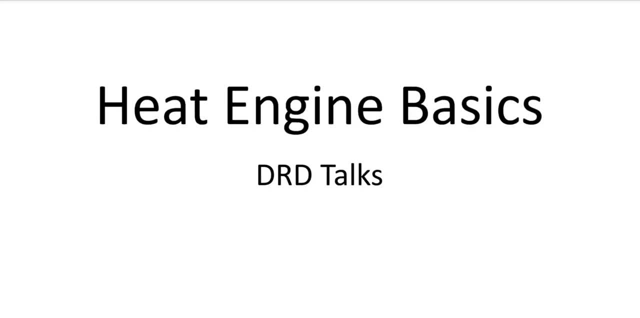 Welcome to all in this lecture. From this lecture we are starting a new series, The series of basic engineering. In this series we are going to deal with basic mechanical engineering, basic civil engineering and also the basic electrical engineering. We are starting with the mechanical part. In this mechanical part we are going to study the heat engine basics. Before studying the heat engine basics, we also need to have the knowledge. 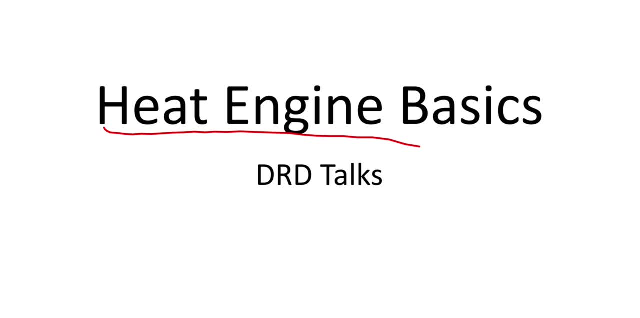 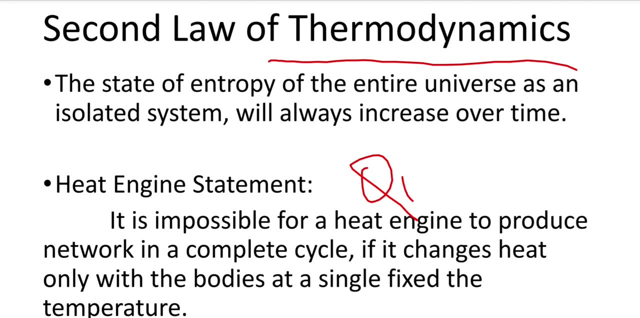 of second law of thermodynamics. So let's see what the second law of thermodynamics state. The second law of thermodynamics is also known as the law of quality of a system- Quality of a system, or it is also known as the entropy of the system. What is? it is also known as the law of entropy of the system. So let's start. It is the statement, the state of entropy. What does the word entropy means? The palace. 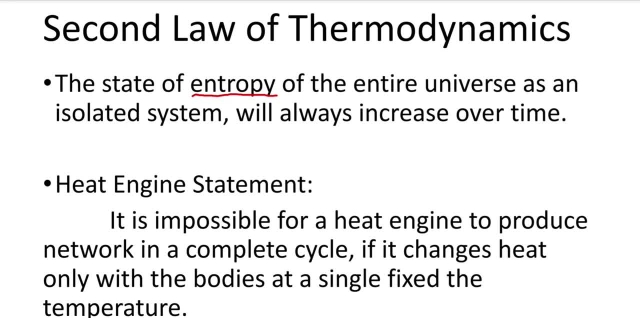 word for entropy can be: randomness Means the amount of motion that a particle deals with. It is known as the entropy. More the energy, more the entropy increases The state of entropy of entire universe. as an isolated system Means the heat is not exchanging from the universe, There is no radiation. Temperature is not decreasing In such an isolated system, as an isolated system will always increase over time. 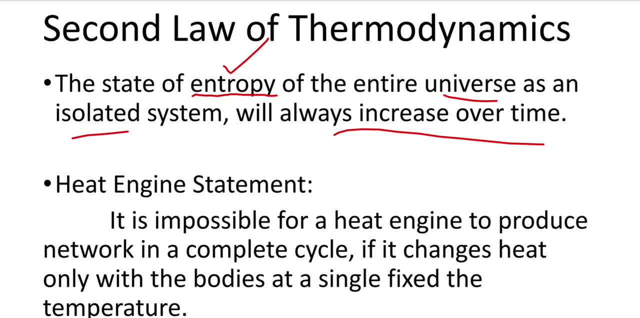 Means the heat in the universe will always increase, It will never decrease, It will always increase. As time goes on, the heat will increase. If we deal with the heat engine statement, The statement of second law of thermodynamics, From the heat engine point of view, What does? it says It is impossible for a heat engine, Impossible for a heat engine, to produce a network in a complete cycle. 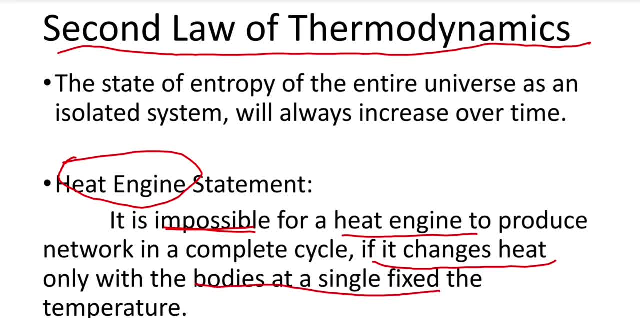 If it changes heat only with the body at a single fixed temperature. What does it mean? In a single cycle Means when the piston is there. That BDC means from the bottom dead center Will go to the top dead center And will come back to the bottom dead center In that complete cycle. 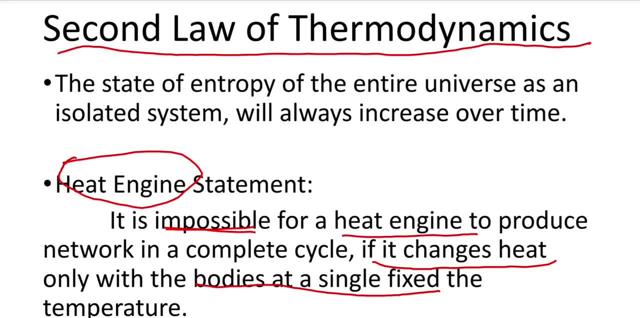 It does not exchange heat only once There are many heat exchangers. OK, What is written here? Impossible Means it is not possible that the heat engine will only exchange temperature once in a cycle. This is what the heat engine statement says. OK Means its more If we look at it from the point of view of the second law of thermodynamics. 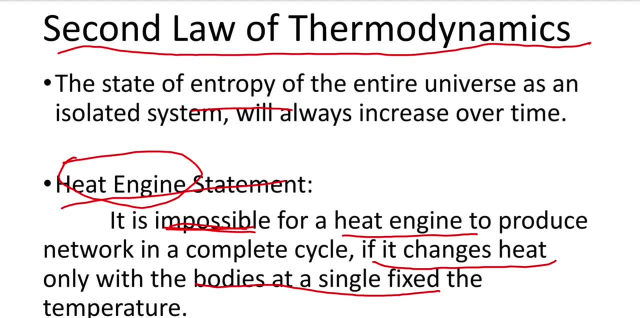 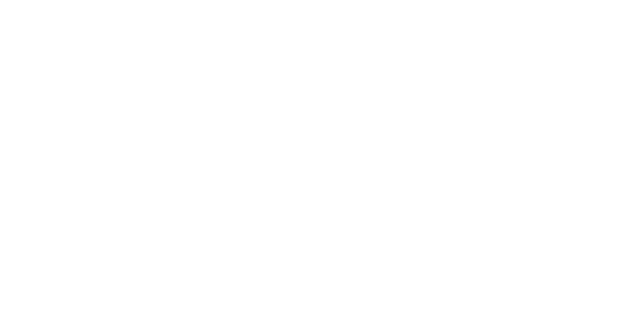 That entropy will increase, But not at a fixed temperature. That temperature will keep on varying. So let me tell you an expression: Efficiency of a heat engine is equal to work upon heat. OK, Efficiency, What can we call it? It is a parallel statement, It is a parallel equation to the second law of thermodynamics. 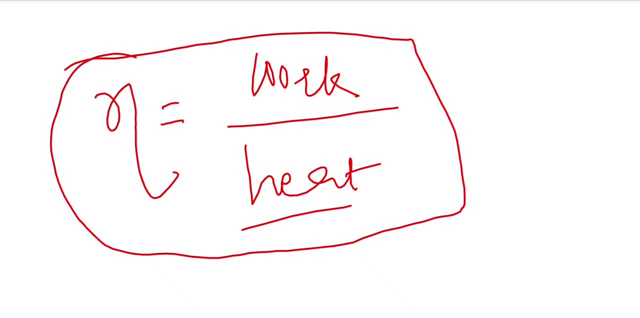 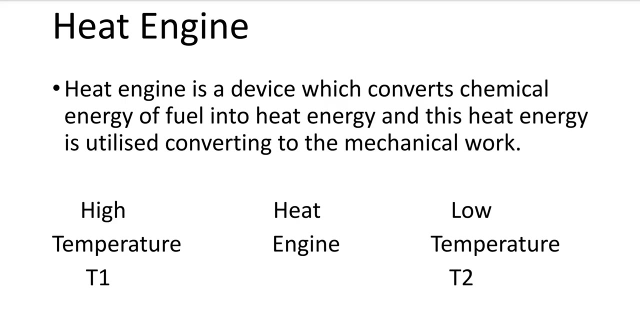 What does it say? Efficiency, eta is equal to work Upon heat transfer. OK, This is what our equation says. So let's go ahead. Let's see the heat engine now. This is a basic lecture Here. we will not cover the heat engine in more depth. 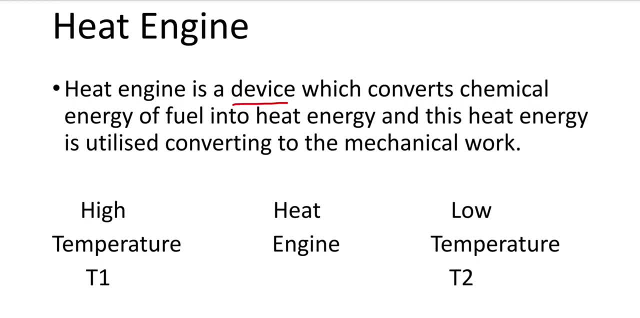 So heat engine? Heat engine is a device which converts chemical energy of the fuel into heat energy And this heat energy is utilizing, converting to the mechanical work. OK, Let me give you an example of this. Our car is running On which On the fuel. We consider the fuel as the petrol. 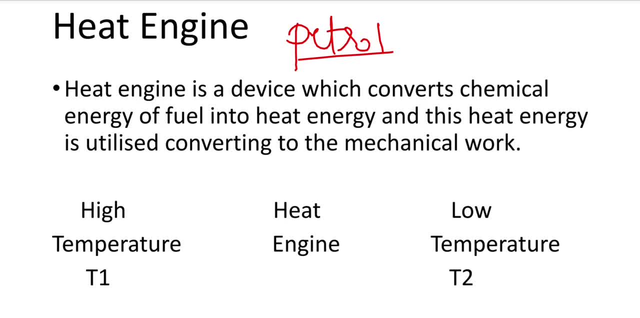 OK, We have set the petrol on fire, Means what happens: There is combustion in the engine, Means the petrol is on fire. So then the conversion of that petrol will be in the heat energy. It is obvious that when the petrol burns then the heat comes out of it. 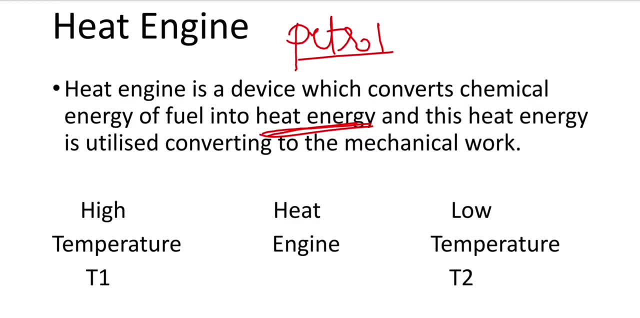 Converted to heat energy. And now, what did we do? That heat energy which was generated in the cylinder, That heat energy covers the piston back, Due to which the crankshaft rotates. And when the crankshaft rotates, then the power is received. 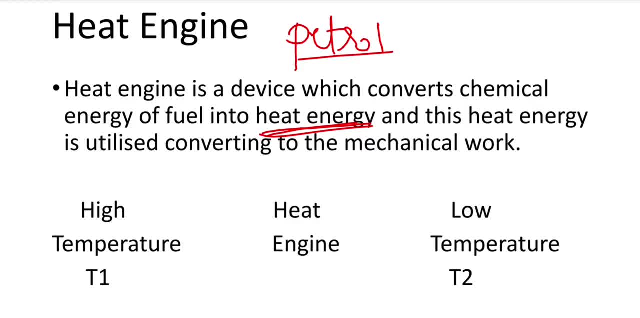 And due to which the car runs. Means what happened Converted to mechanical work. OK, So let's see What happens first. This is a basic diagram of our heat engine. OK, OK, So what happens first? This is a basic diagram of our heat engine. OK, 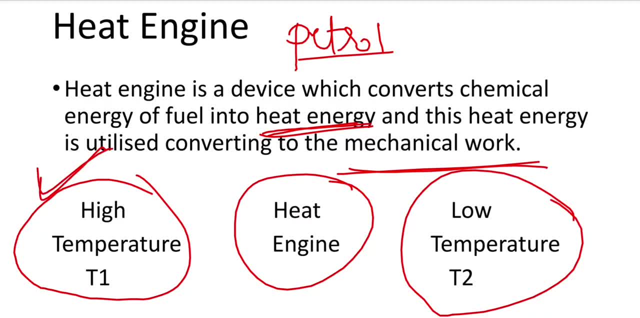 There are three components in it. There is a high temperature source, From where the heat goes to the heat engine. The heat engine gives mechanical work. while using the heat, It produces some work, And the remaining heat goes to the low temperature reservoir. 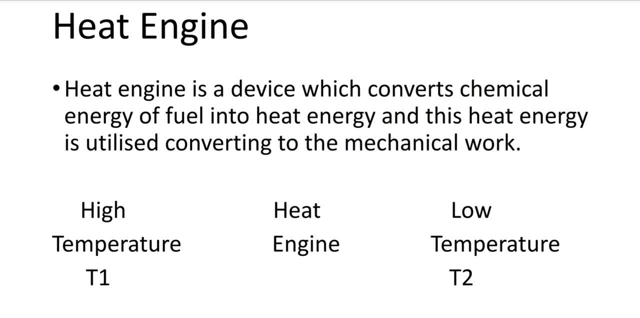 So let's see it properly. High temperature T1 goes to the heat engine through a thermal energy source. It supplies Q1 amount of heat to the heat engine. OK, When this heat engine gets this Q1 amount of heat, Then this heat engine gives us some W work. 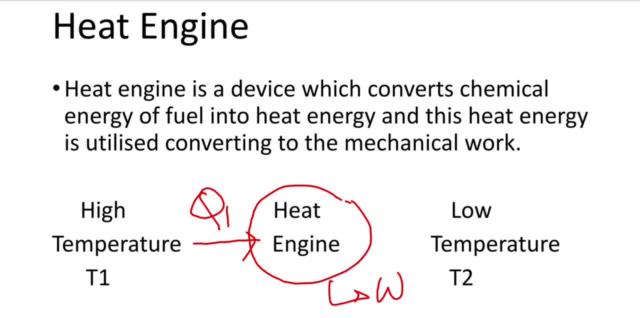 We get some W amount of work from the heat engine And the remaining heat. Why will there be remaining heat? Because there is no such engine in this world Which has the efficiency of unity. We cannot get the efficiency of unity Every time the efficiency is less than 50.. 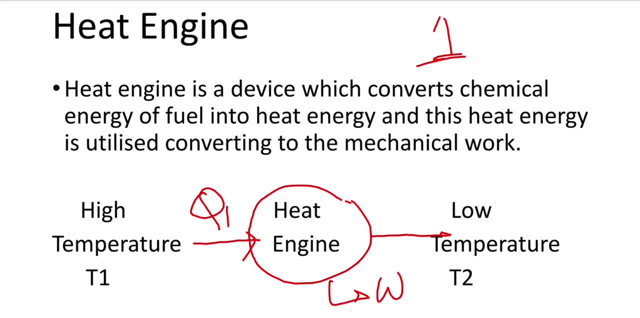 And the maximum is less than 40.. OK, The efficiency cannot be unity. This machine is not made. OK, So some heat will be lost. We call it Q2.. OK, The heat is rejected. This rejected heat goes to the low temperature reservoir. 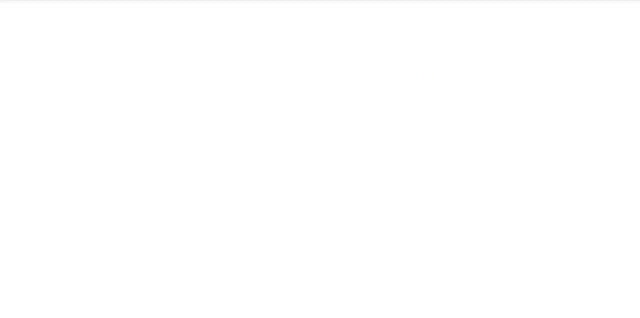 So let's see some basic expressions for the heat engine. First of all, efficiency is an important term. Efficiency is shown by eta Efficiency, eta, is equal to work net upon Q1.. What is Q1? Heat supplied. OK, This Q1, how can we write it? 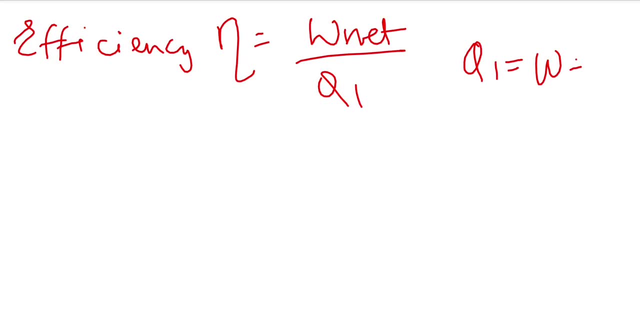 W, amount of work comes from Q1. And what is Q2?? The amount of heat is wasted. That means Q1 is equal to W plus Q2.. Then what will come if we remove the value of W from this equation? W is equal to Q1 minus Q2..